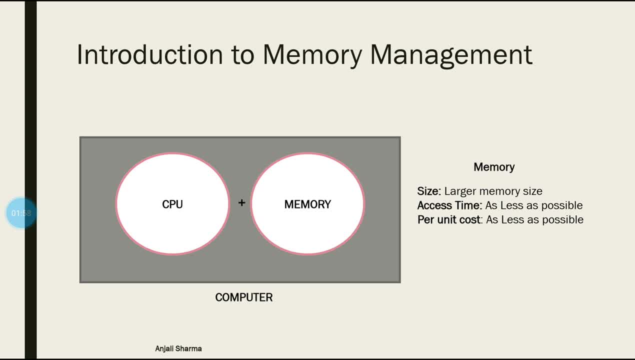 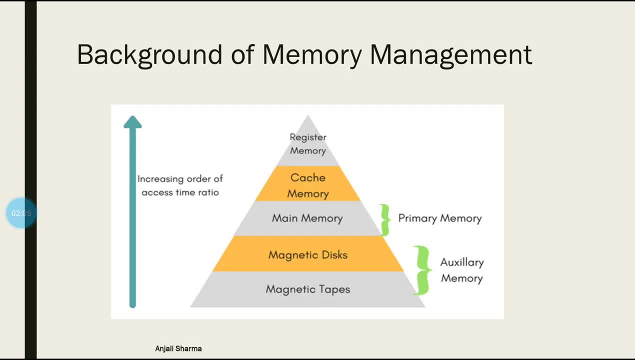 characteristics is not possible. So what we have generally seen in our computer system is a different hierarchy of memories that is given in this particular figure. For example, we have an auxiliary memory or secondary memory, which includes the magnetic disc and the magnetic tapes. Now, talking about there, excess time is very large, Excessing the data from secondary memory. 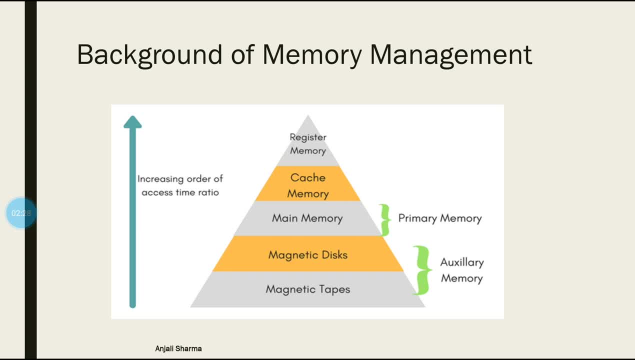 takes considerably a larger time time as compared to your primary memory. so a certain type of memory which is magnetic, in order of execution right, is considered as the secondary memory, which is our disk drives. then the next hierarchy is the primary memory or the main memory right now, as per the cost. 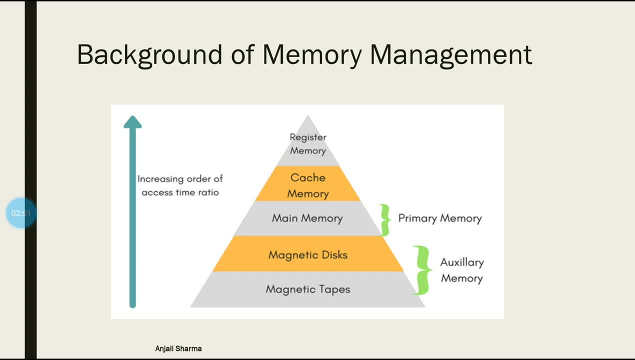 the cost increases as we moves up in the hierarchy and the excess time decreases. so main memory has a direct access to cpu. therefore the excess lag is slightly reduced as compared to your secondary memory and the cost becomes higher. then we have the upper hierarchy memory types, that is, the cache memory and the resistors. resistors are uh, reside with 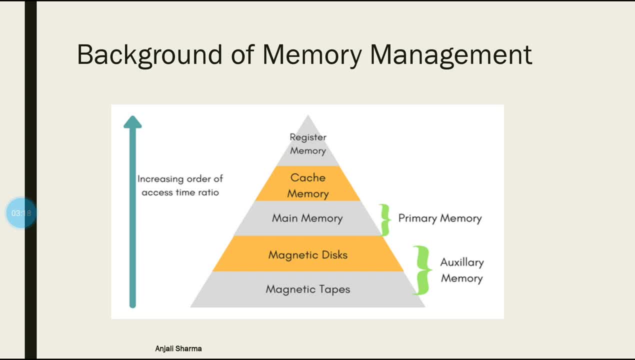 the cpu. cpu can have direct access to both the resistors and the cache memory, and the concept of cache memory is that the frequency of the memory is the frequency of the memory and consequently, excess data is put into the cache memory so that the excess time reduced. 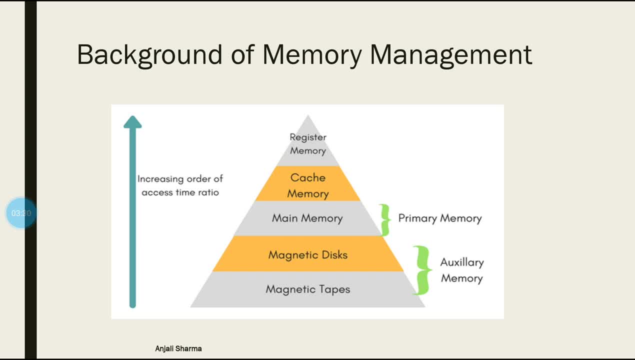 on furthermore, right. so basically what happens? this scenario: you guys have also noticed that when you buy a desktop or a laptop, you can considerably notice the size difference between the hard disk and the ram. you get the hard disk, you get about 512 gbs or 1024 gbs, but 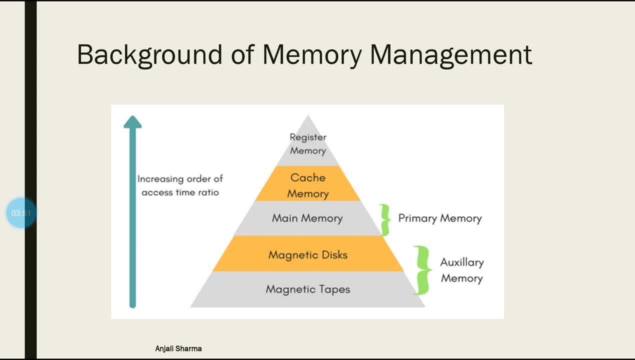 as far as the ram is concerned, the size is not more than 4 gb or 8 gb, right, because the ram is costlier and have less amount of storage, right? so basically what we did? we just fragmented our memory into different types. we also have a concept. 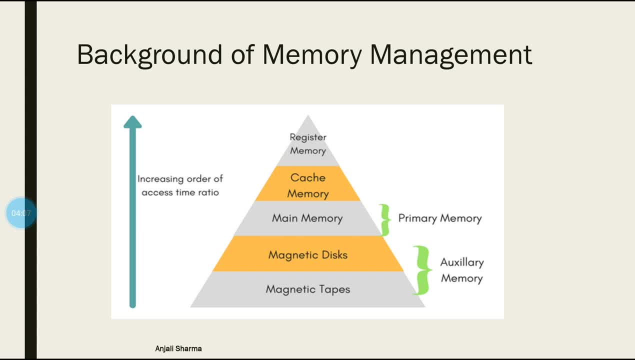 of virtual memory, which we will be discussing later on, but till now, you need to understand that the memory is divided into different types based on their characteristics. it can be auxiliary memory, primary memory and, of course, your cache memory and your resistors. right, talking about the background of the memory management, it is something like that that 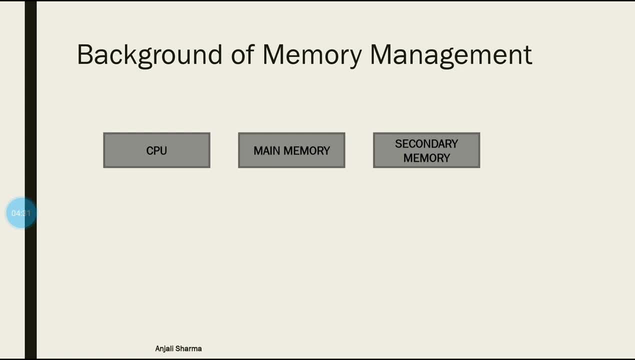 cpu main memory and the secondary memory comprises of your computer system as a whole. right, and the work that will be done is as follows. the first task is which data from the secondary memory should come to the main memory and at which location. so here what we need to. 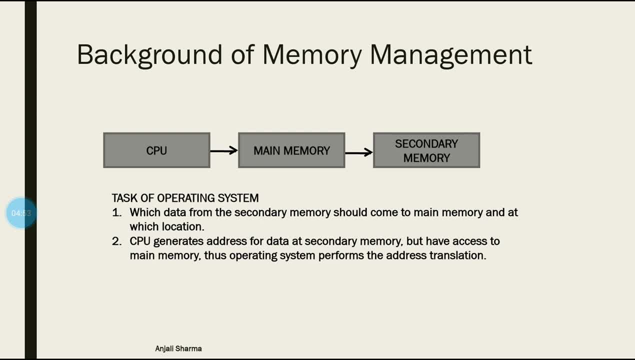 understand is that when we store a data, we store that data in the disk right and the data is to be transferred from your disk to your main memory so that the cpu can access it. you can see the diagram that the main memory has direct access to your secondary memory and your cpu has a direct access to. 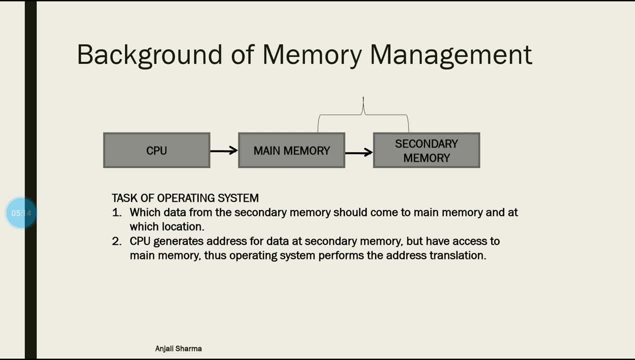 the main memory. therefore, what you have to do, the data from the secondary memory has to be transferred in the main memory so that the cpu or the processor can access it right in these migranes supermercial processor's memory. but we can get the main memory via cpu. but the cpu doesn't havegemean iPhone or cpu abilities. right same. 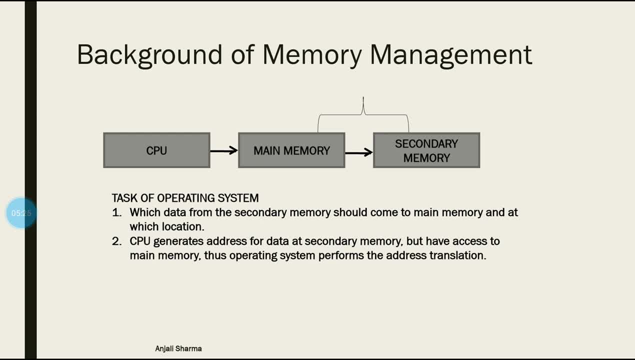 So the first task that operating system does is to decide when and which data from the secondary memory is to be transferred to the main memory. The next task is: CPU generates the address for the data at the secondary memory, but it has access to the main memory. therefore, operating system has to perform this address. 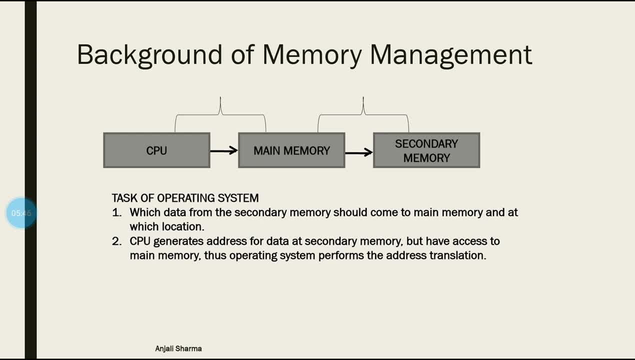 translation. Now the address is generated by the processor and that processor generates the address. you must have studied in computer organization that there is an address register which has the address of the various instructions or the program. So now that address belongs to the address of the program in the secondary memory. but 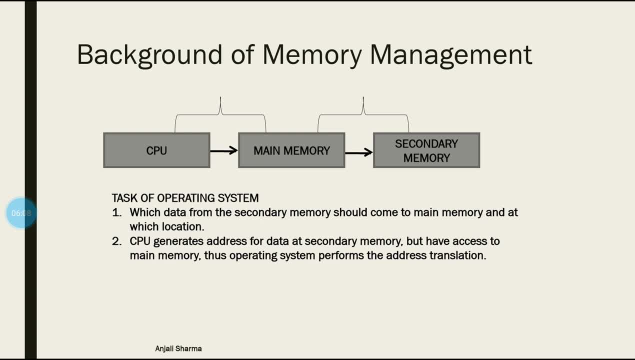 the CPU cannot access the secondary memory. it can access the main memory. therefore, the mapping or the translation of the address should be placed right So that task is also done by the operating system to. during the course of this unit, you will be studying how the